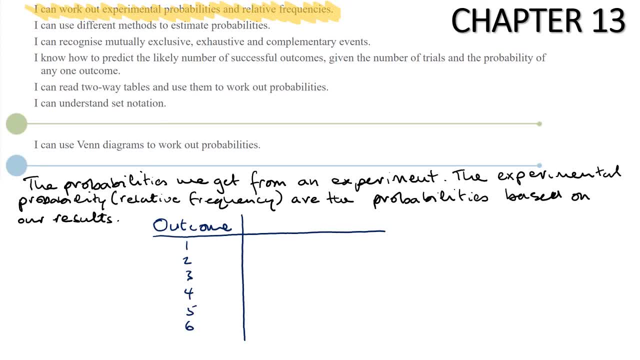 And in the second column I'm going to put the frequency. So this is basically how many times this value came up. So how many times would we expect them to come up? Well, we'd expect each one to come up 20 times. 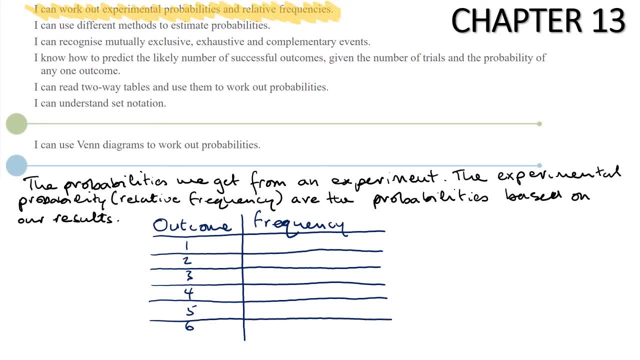 That's what we'd expect. Is each one going to come up exactly 20 times? Maybe, maybe not, But when we do experiments, things do vary from what we expect them to be. So let's say the 1 came up 17 times. 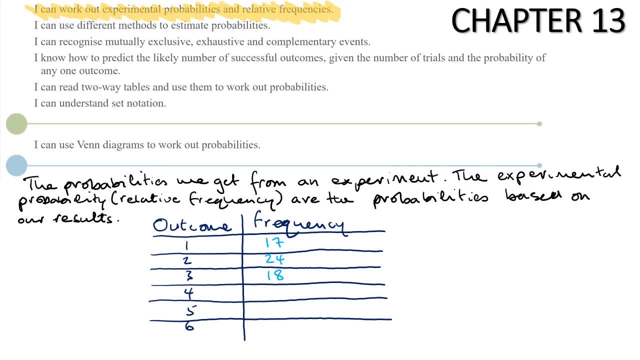 The 2 came up 24 times, 3 came up 18 times, 35 times for the 4., 4 times for the 5 and 22 times for the 6. And all of these added up make 120, because we said we're going to do it 120 times. 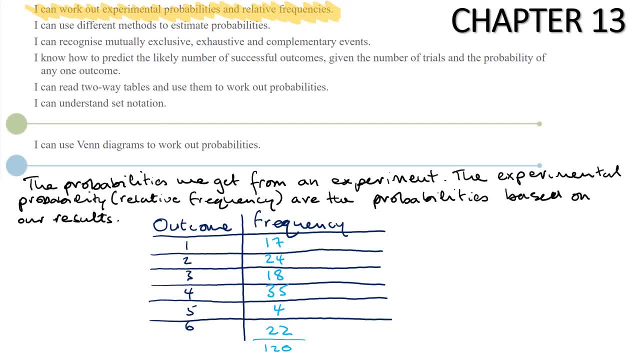 And the probabilities we get from these can be called the experimental probability or the relative frequency. These would be so for the first one it would just be 17 over 120.. The second one would be 24 over 120.. You can simplify if you want. 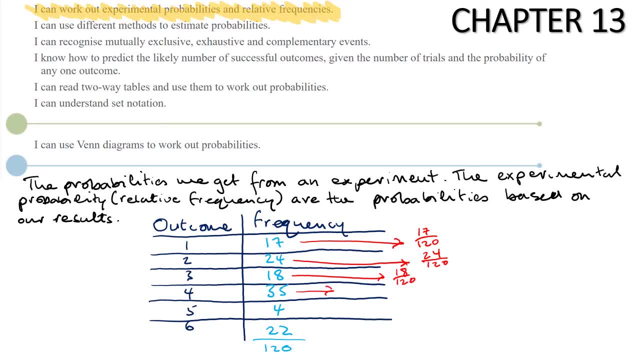 Then 18 over 120.. 35 over 120.. 4 over 120. Or 22 over 120.. So these probabilities that we have here, that we've got written down, these are what we call the relative frequency or the experimental probability. 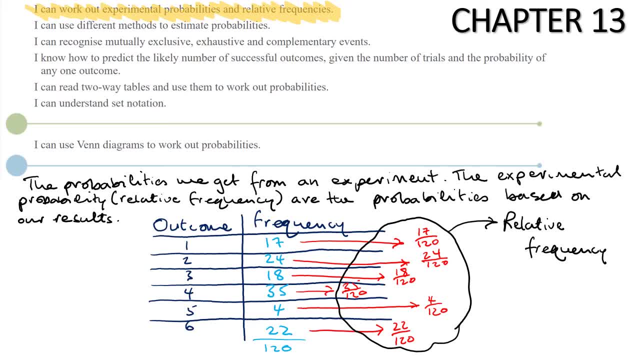 Yeah, it means the same thing. Now, looking at this table, we could probably look at it and say, hang on, it looks like this dice might be biased because look, 35. 4.. One of them seems a bit high. 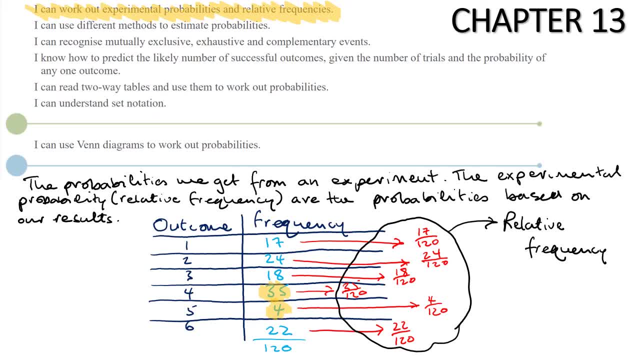 One seems a bit low. So we can use what we expect to happen and compare that to the relative frequency or compare it to the frequency and decide whether something is biased. So we can decide if something is biased, Something is biased, By comparing our results. 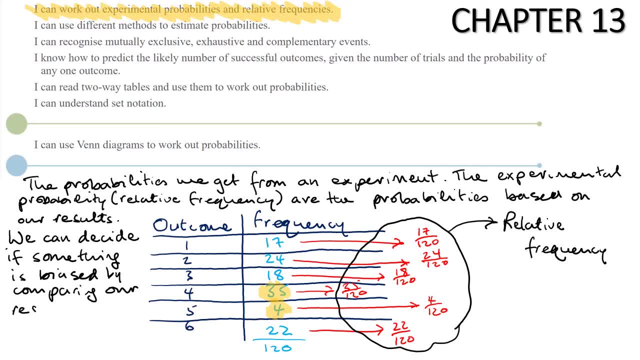 comparing our results with what we expect to happen, And what we expect is that each one of these should be around 20.. As I said, it may not be exactly 20, but if something is way higher or way lower than 20,. 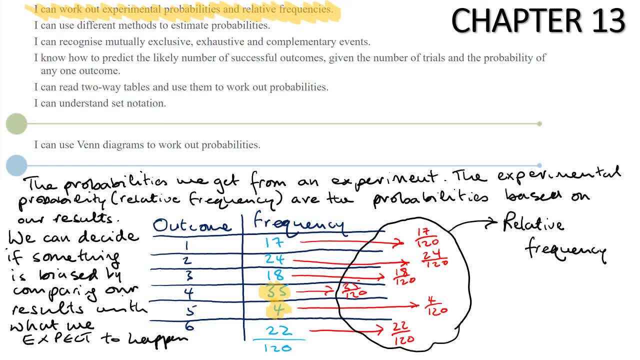 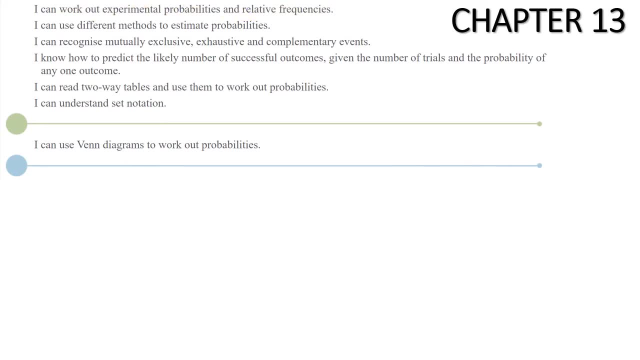 we expect. you know that suggests something isn't right, So we might use the word biased. So we should be able to decide something is biased by looking at the results we get from a table Right? The next thing we've got on our list here is: 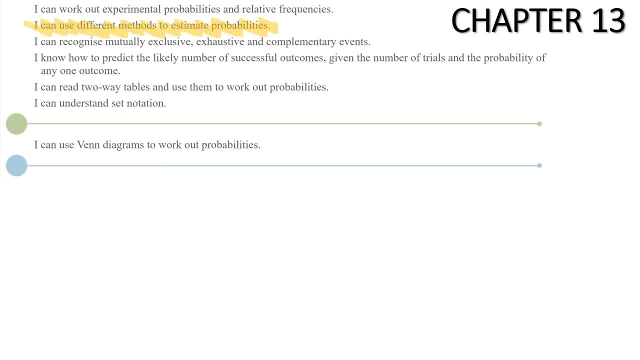 using different methods to estimate probabilities. Okay, Now, this is basically predicting how many times. how many times, just as we said before, we expect something to happen. Now that might be dice, it might be coins, or it might be. we're given a question like this: 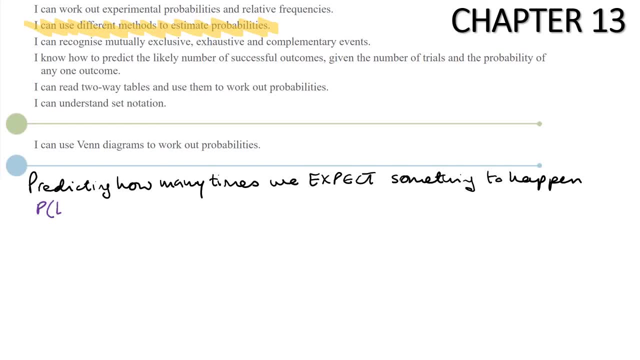 We're told that the probability of heads is 0.7, which means the probability of tails must be 0.3.. We'll talk about that in a minute, why we know it's 0.3.. And let's say that we had a coin. 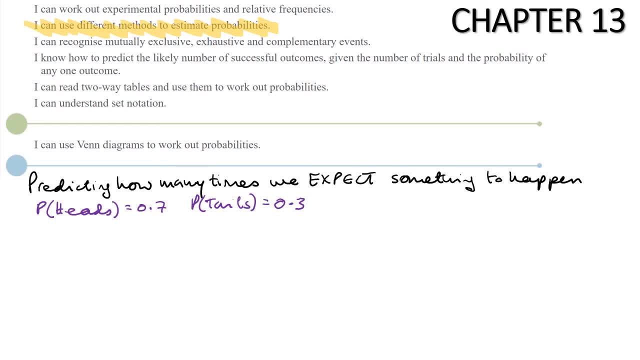 and the coin is flipped. Coin is flipped, Let's say, 60 times. Can we predict or estimate how many times it should come up heads or tails? Well, all we do is we take the probability and we multiply it by the number of times. 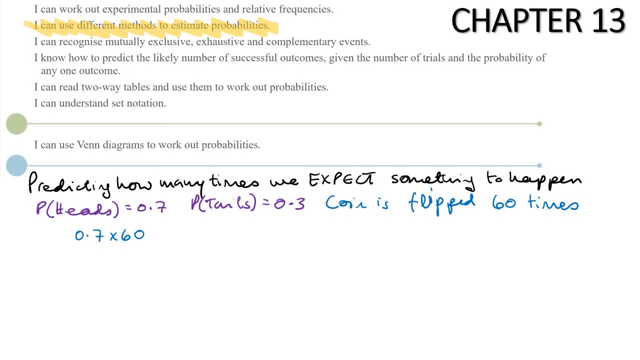 that thing has been done. So if I do 0.7 times 60, I get 42. So I expect 42 times it lands on heads. And then if I do 0.3 times by 60, actually I could even take 42 away from 60,. 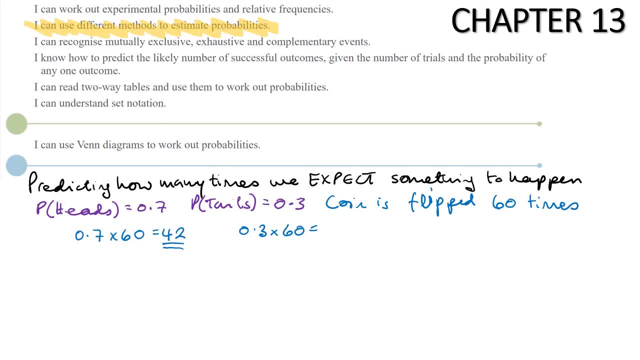 couldn't I to work out what's left. I get 18.. So I would expect 18 tails to come up Now. all we did there was we took the probability and we multiplied it by the number of times this thing was done. 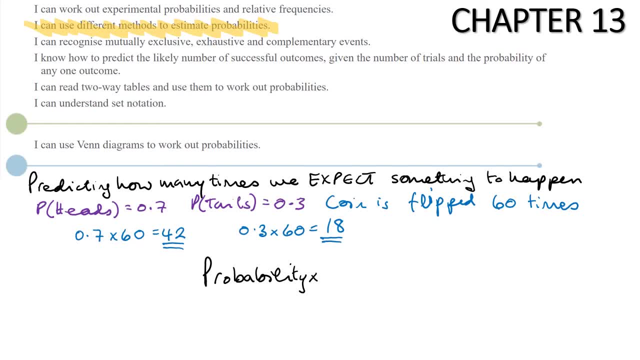 I'm going to call it the number of trials. Number of trials, Now. what I mean by the number of trials is basically how many times is this thing or event being done, Or how many times is this thing going to be done in the future. 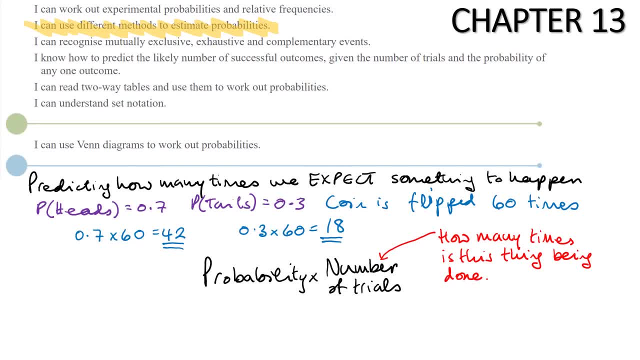 But the important thing is you take the probability of that thing, you multiply it by the number of trials, the number of times it's being done. That might be the number of days, might be the number of flips of a coin, could be anything like that. 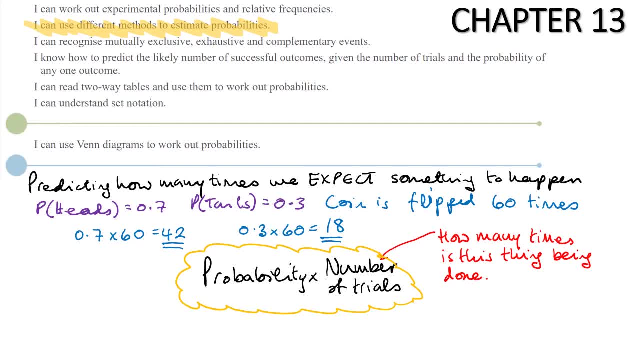 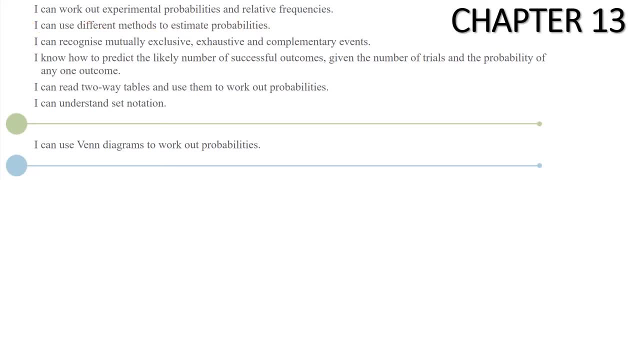 You multiply the two together and that gives you an estimate of how many times you expect that thing to happen. Right, the next thing we've got there there is mutually exclusive, exhaustive and complementary events, So let's go through all three. These are like definitions. 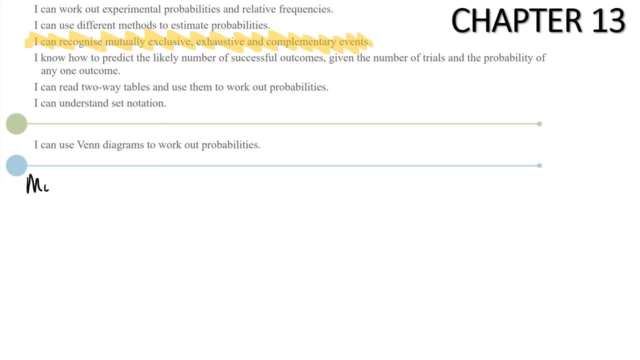 So the first one mutually exclusive. Mutually exclusive Right. this is basically means that these are two events that cannot happen at the same time. Could be more, but normally it's two events that cannot happen at the same time. Example: 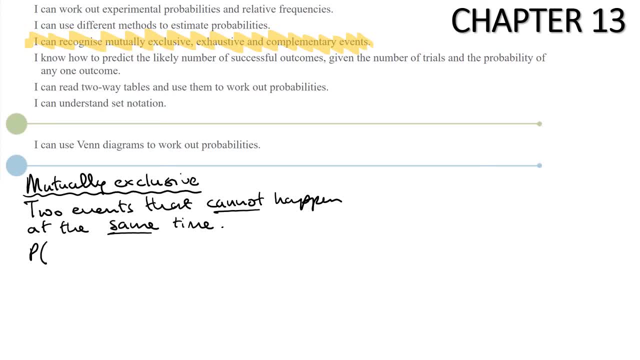 The event rolling an even number on a dice. Not the probability, but the event. The event rolling an even number on a dice And rolling an odd number on a dice are mutually exclusive. They can't happen at the same time. You cannot roll a dice. 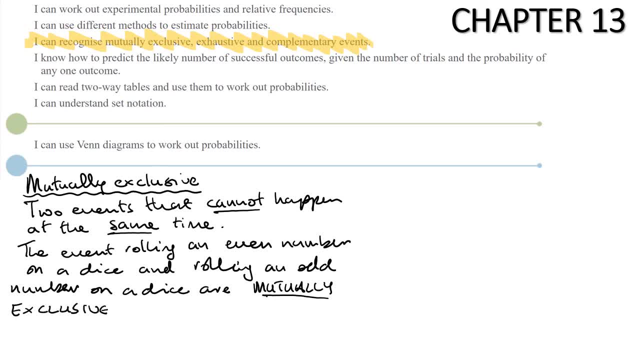 and get an odd number and an even number at the same time. So we describe them as mutually exclusive. So these are things that cannot happen at the same time. Exhaustive, Exhaustive, Exhaustive. Okay, now this is a list of all the outcomes. 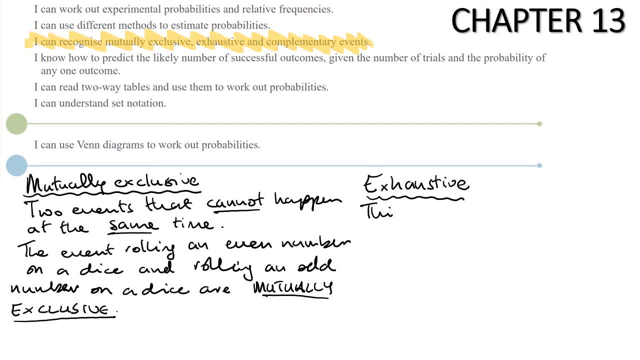 all the things that can happen. Okay, so this is a list of all of the outcomes, And what's special about it is that all the probabilities of all these outcomes will add up to one. Okay, so I'll put there: probabilities add up to one. 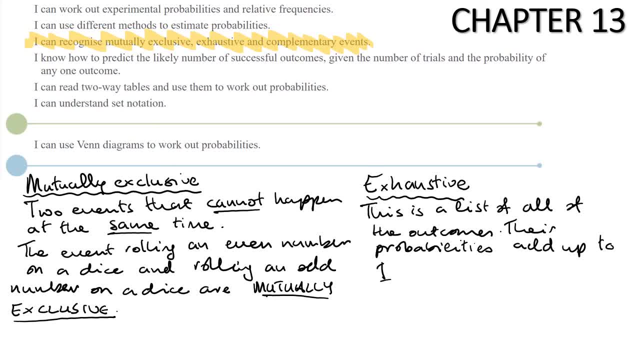 So, for example, let's say I flip two coins And the options are: I get heads and tails. So I'm just writing a bit of shorthand here: Tails and heads, Tails and tails, Or heads and heads, So you can see. 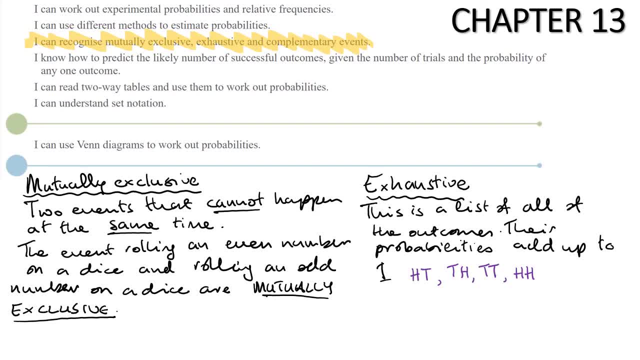 there are four different sets of things that can happen. This is an exhaustive list because it's everything that could happen. Okay, When you have an exhaustive list of things, you've basically written down everything that could happen. So that's an exhaustive list. 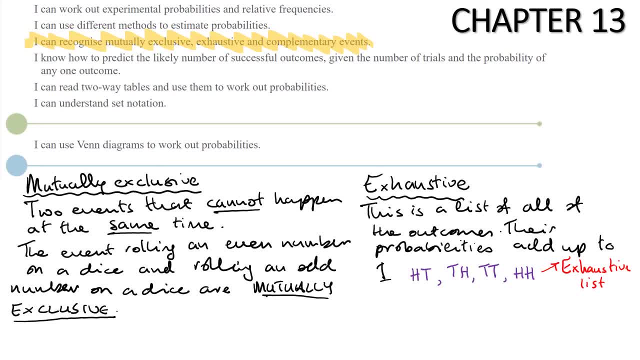 What can happen. The probabilities of each one of those things happening is a quarter And if I add those probabilities together we get one. So when you've got an exhaustive list of outcomes of things that can happen, when you add their probabilities together, they always add up to one. 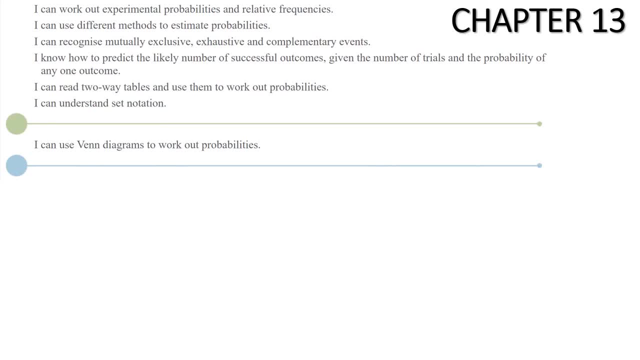 And the last thing on that list was complementary events, And we've used complementary events without even thinking about it. When we were looking at the probability of heads and tails, I told you what the probability of heads was. You knew what the probability of tails is. 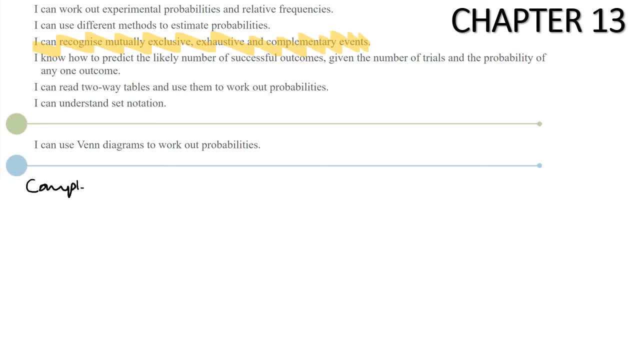 Complementary events, Com-ple-mentary events- They're these things where you've got two paired events where one is something happening and the other one is the same event not happening. So complementary events are paired events whose probabilities add up to one. 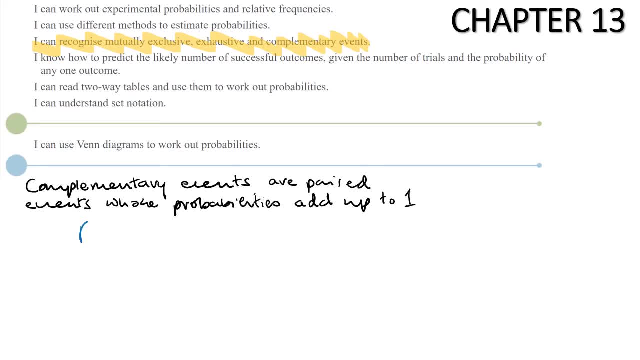 And we use it all the time. So, for example, if I had a question that said the probability it's going to rain is 7 over 10.. What's the probability? It's not going to rain. So notice, I'm just using shorthand here. 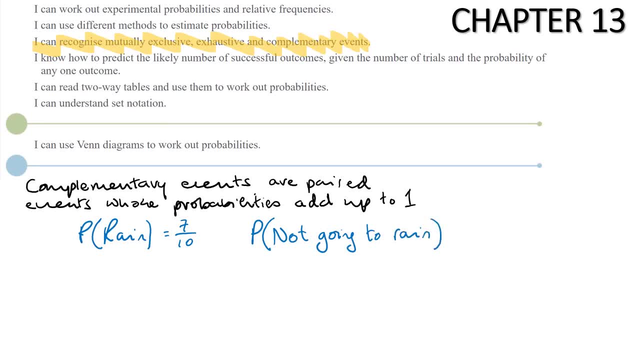 probability in something in brackets, or p with something in brackets, just means the probability of. we know this is 3 out of 10 because these are complementary events- One is rain, one is not rain- And complementary events they're like these paired events whose probabilities add up. 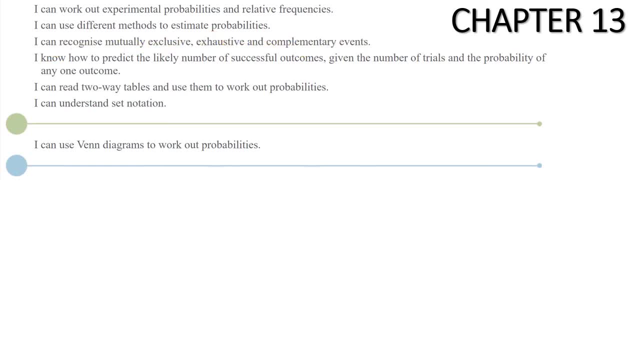 to one Right now. the next bit here we've sort of already talked about when we've looked at estimating probabilities and things like that. So the next thing we're going to look at on this list is these two-way tables. So this is the next thing. 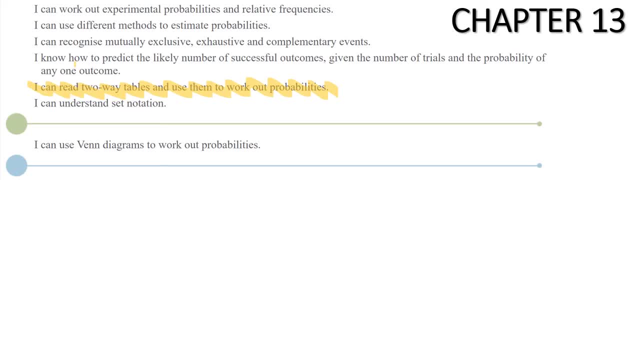 we're going to look at two-way tables and using working out probabilities from them. So here's an example of a two-way table. So let's say this is about boys and girls in a school and those that walk and don't walk to school. 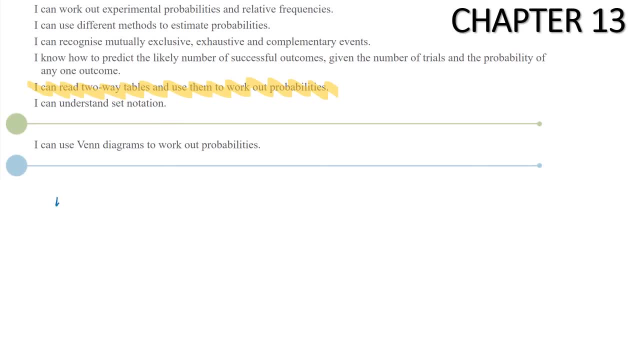 Okay. so let's say, walk here, don't walk like this, and we'll put this in this two-way table like this. so along the cross top here I'm going to put boys and girls like this. Now, these two-way tables always have like a column. 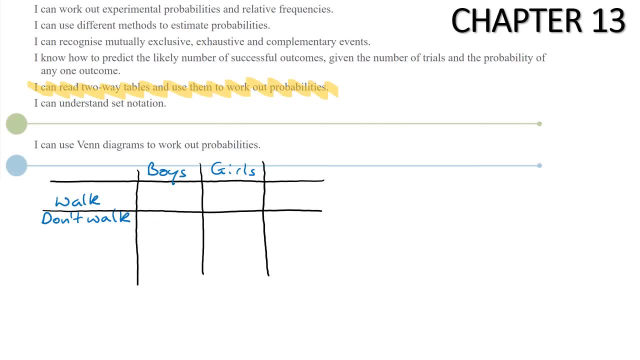 which is the total. So we're going to have a total here, We have a total down the side and you have a total along the bottom Total here, And we're going to fill this in Now. quite often in questions like this they're partly filled. 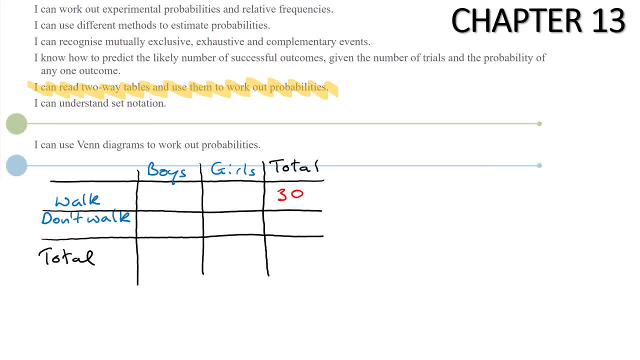 in and you need to fill in the rest. So let's say that this was given like this and it might say something like: I don't know. there are four more boys than girls, So we're going to use this information to fill in the table There. 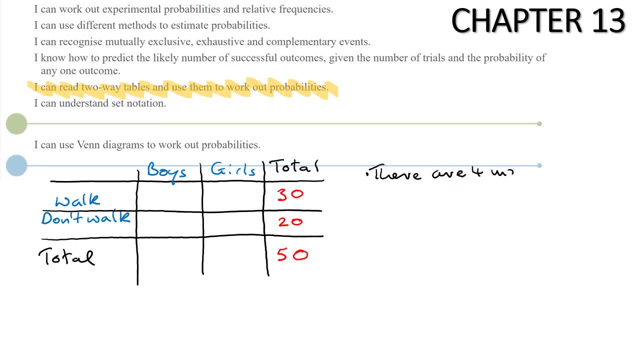 are four more boys than girls. Now I know that the boys and girls need to add up to 50.. Now the numbers that are going to make that work is 27 here and 23 here. There's four more boys than girls and that adds up to 50. 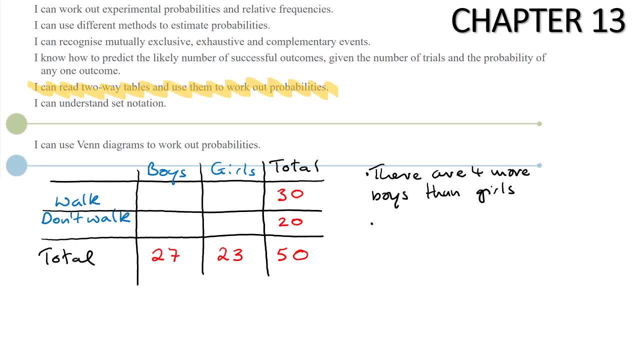 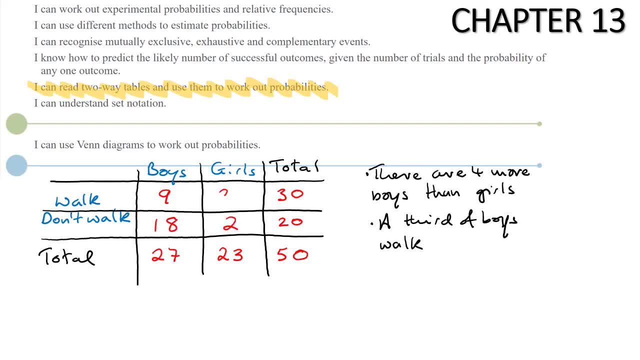 which means that this number here must be 18, and then it's all slots into place. This must be 2, and then this must be 21.. Yeah, So everything should add up to the right things. Now I can work out all sorts of probabilities. so let's say I wanted to. 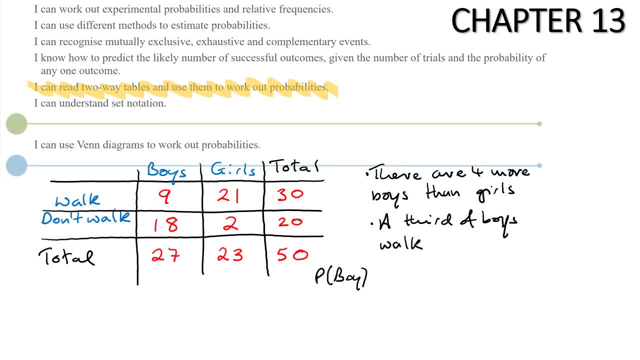 work out the probability that they're a boy. Well, I can see there are out of 50 altogether. what if i want to know the probability that they don't walk, the probability that they don't walk? well, those that don't walk, there are 20 of those out of 50.. 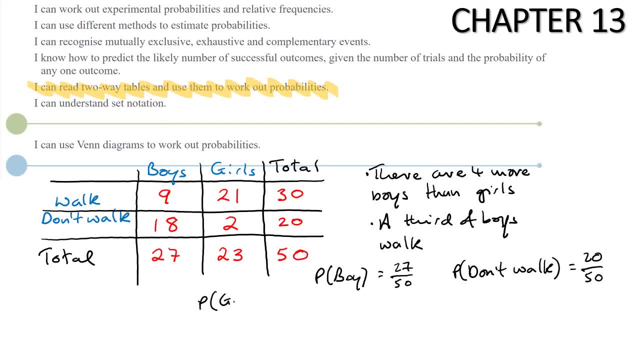 what if i wanted to know the probability that there are a girl that walks? a girl that walks, okay, so the girls that walk. there are 21 of those out of 50. something at the high level might be a question like this: um what? oh no, not, not what, but given that, 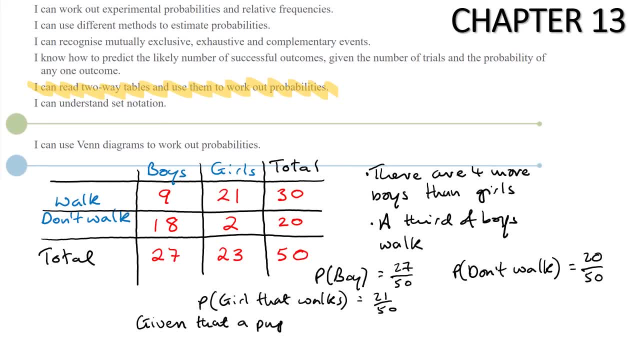 a pupil is a boy. what is the probability? what is the probability they walk? now this wording is slightly different in it and the important bit is this: given that the pupil is a boy, now if we're telling, telling the person already the person is a boy. that means: 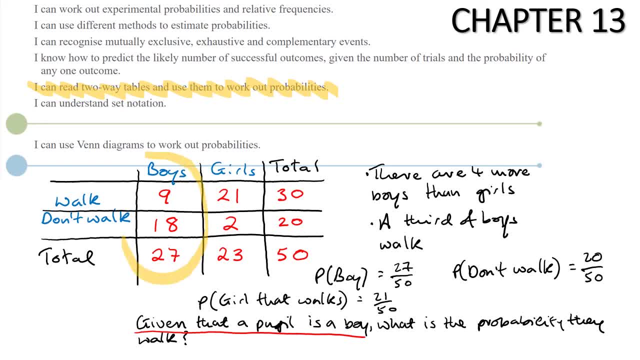 it is only. we're only looking at this part of the table. yeah, we are not looking at anywhere else in the table. we are already told that they're a boy. now, if that's the case, it's going to be. this probability is going to be just. 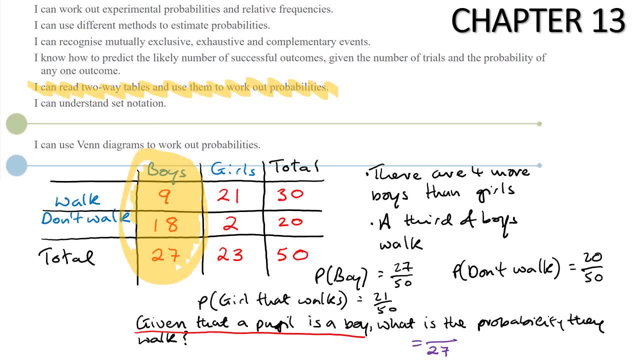 out of 27.. so we're already told the fact. given that the fact that they're a boy, so it's only at 27.. now, out of those 27, how many of them walk? nine, so the probability that they- uh, given that the person is a boy, the probability they walk is just 9 out of 27.. it would not be 9 out of 50. 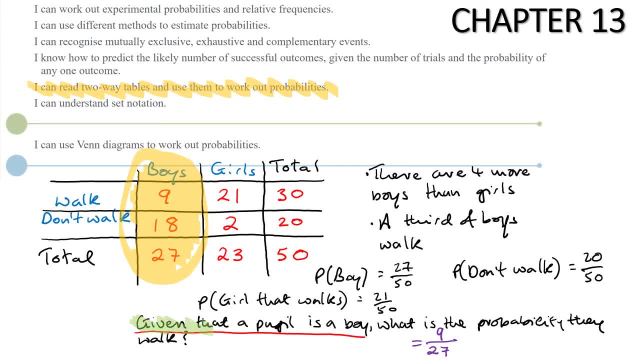 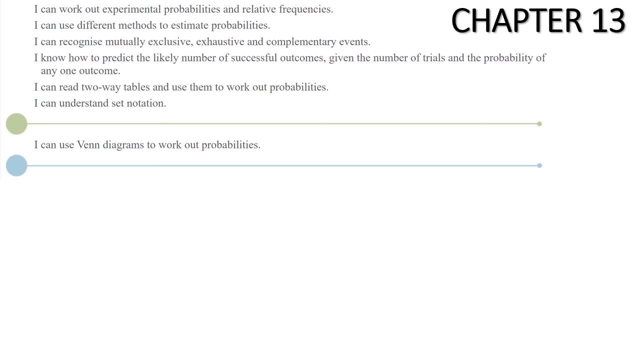 because of this extra bit of information here which makes it slightly different. and that would be at the top end of these probability questions. last thing we're going to look at now is venn diagrams and set notation. that all goes together. so this bit here and this bit here. now the last. 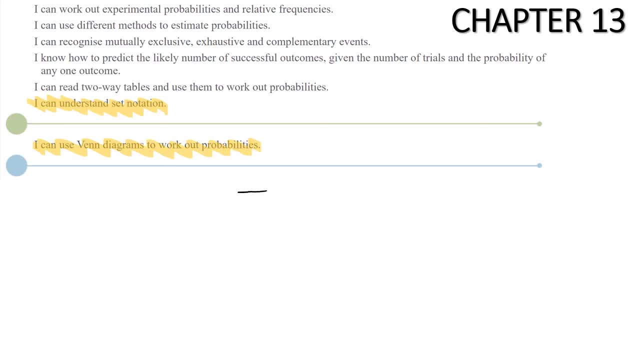 the last time you use Venn diagrams was for lowest common multiple, highest common factor. so with Venn diagrams you normally have like a rectangle like this. that rectangle is called a sample space. you may remember sample space diagrams, so that's called a sample space. every number that we fill in on a Venn diagram. 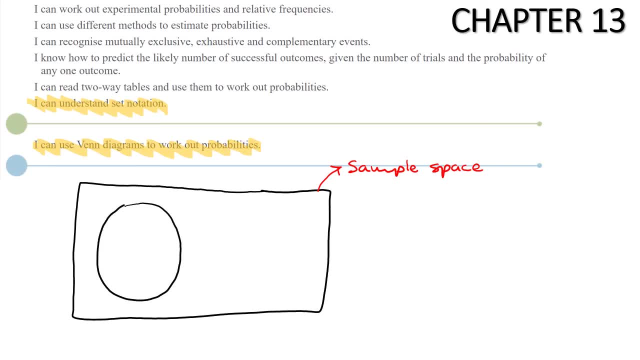 goes into the sample space. you should never be writing numbers outside. okay, so I've got two circles here. I'm going to call them a and b. so before, when we did highest common factor, lowest common multiples, those circles would have had numbers on them and we need to know the name of parts of the diagram. now. this: 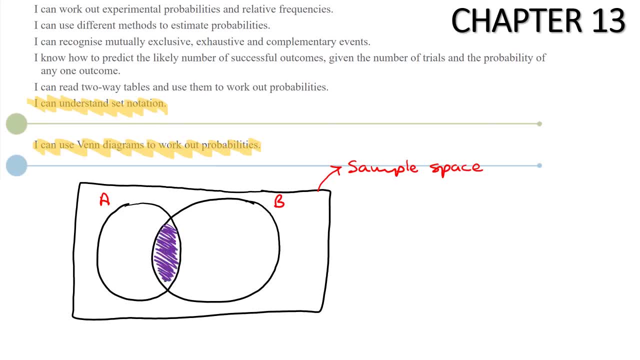 part of the diagram is the overlap of a and b and that part of the diagram diagram we call A intersect B and because we use it so often, we've got a special symbol for its A and then something like that B, so it looks like a C on its side and that we call that A intersect B. so that's that purple part. 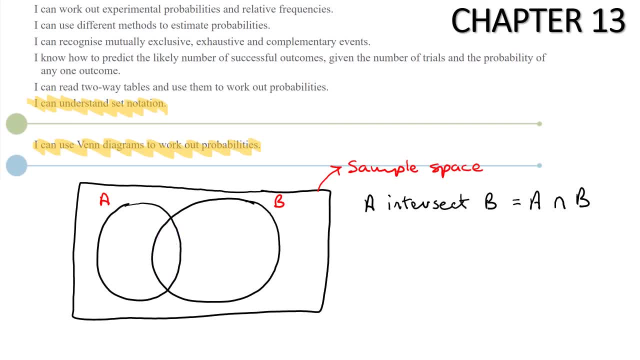 of the Venn diagram. sometimes we need to refer to everything inside both of the circles. so all of this here now that is called A union B, A union B and that symbol is A with a, U and a B like this. so A union B, and sometimes we have a bit. 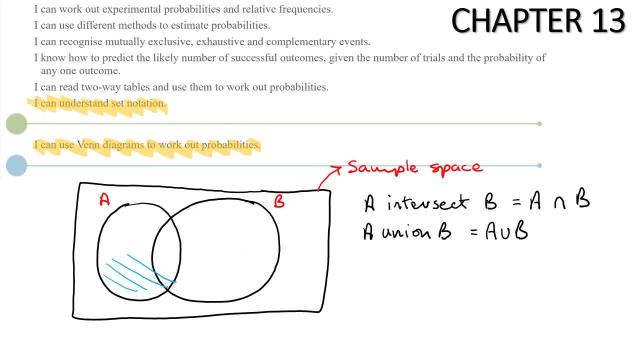 of the Venn diagram, where it's actually something like this: now let me draw this and shade it in. let's use green this time. so if I had something like this, what I'm doing is this is like everything that's not in B. this is everything that is not in B, see I. 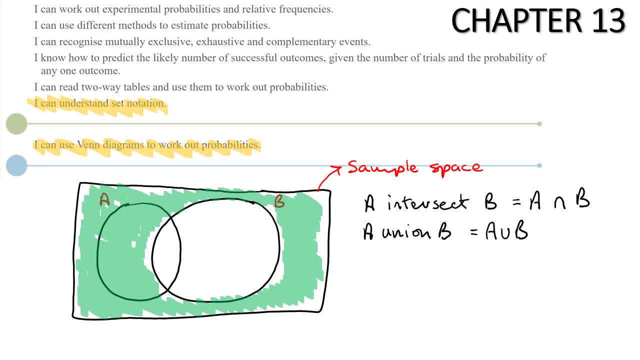 haven't colored in B and we would write that as B with a little dash by it, and we say not B, everything apart from B. now we quite often use Venn diagrams for different problems, so let's change it from A and B and let's change it to cats and dogs. 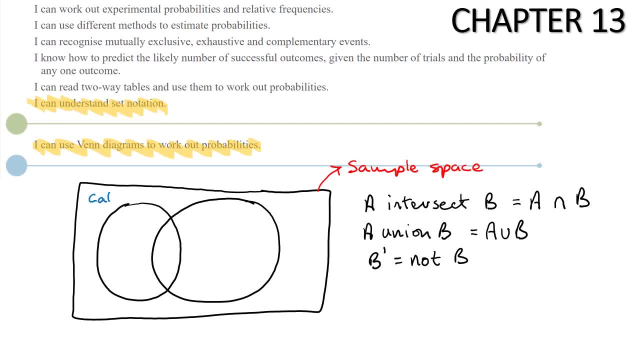 so let's say that one circle represents people that have cats and this circleіс circle represents people that have dogs, and let's say there are 35 people that like cats and dogs. let's say there are 60 people that like dogs. now, I don't put 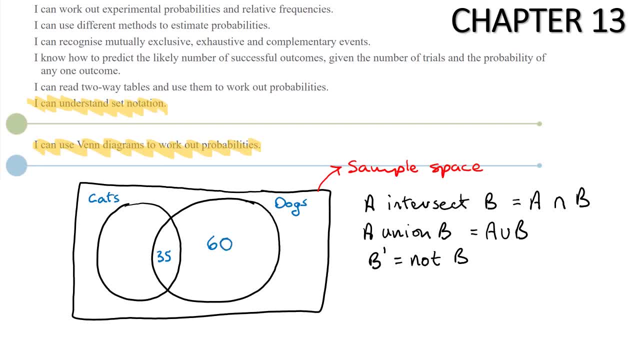 60 here, 60. that's now what I've got. there is 95 people. I've already got 35, so if 60 people like dogs, this should only be 25. inside that circle for dogs there are 60 people. yeah, 60 people like dogs. well, 35 of them also like cats, but 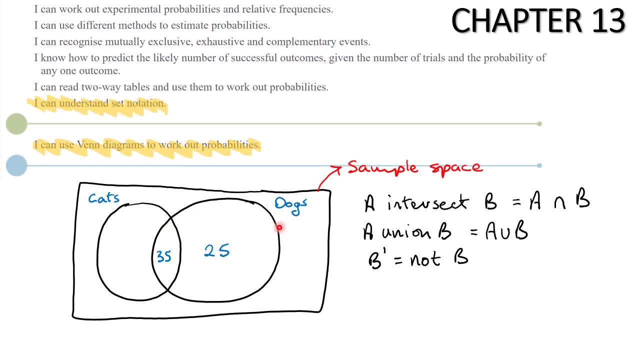 that's 60, so you don't put the 60 in here. in the whole of that circle is 60, and let's say that there are 52 people that like cats. so if I do 52 minus 75, that's minus 75. that would be 25, so that's 25. so if I do 52 minus 75, that's. 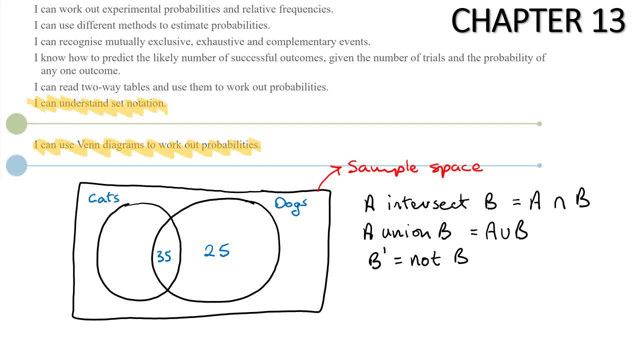 17. so 52 minus 35, I'll get 17 there, and let's say there were a hundred people already we were talking about. that would leave 18 people that don't like cats or dogs. so you do need to be able to fill in a Venn diagram and let's say for: 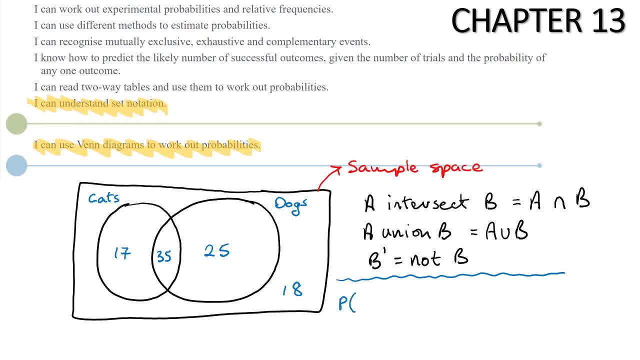 example, I wanted to find the probability that a person liked a cat. that's going to be out of a hundred, because there are a hundred things in there, hundred people maybe that were asked and the people are like cats. that's going to be 17 plus 35, 35, so that's going to be 52 out of 100. let's say I wanted to. 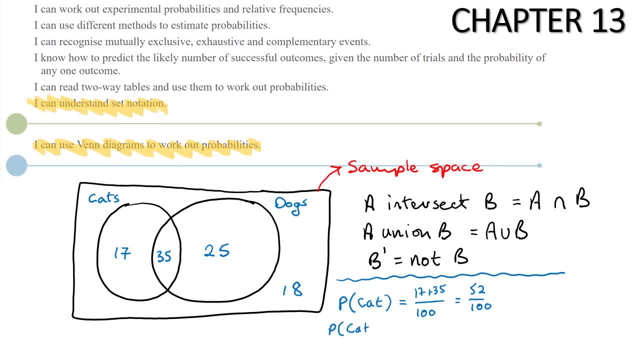 find this a probability: cat, and then that symbol, dog, cat intersect dog. people look like cats and dogs. that would be 35 out of 100. so you can see how we can use this Venn diagram to solve problems. if I want you to find the probability that,